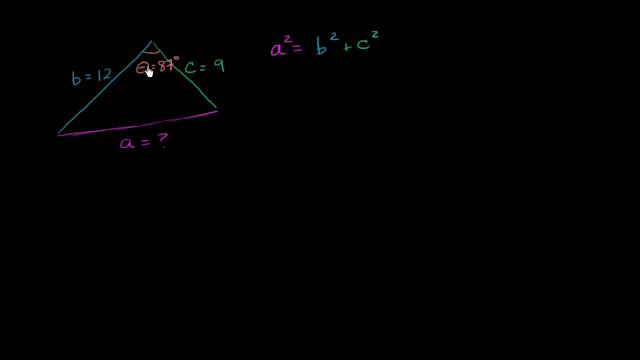 to the Pythagorean theorem so that we can do this for any arbitrary angle. So the law of cosines tells us a squared is going to be b squared plus c squared minus, 2 times bc, times the cosine of theta, And this theta is the angle that is. 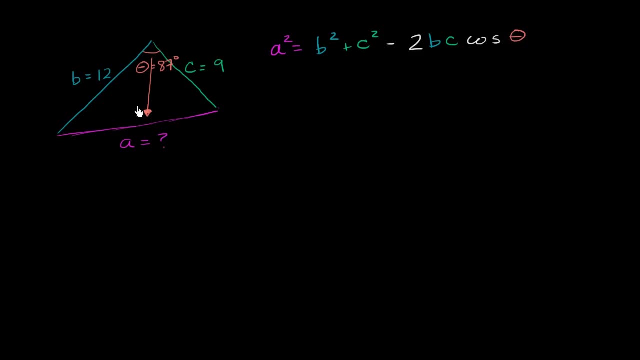 that opens up to the side that we care about. So we can use theta because we're looking for a. If they gave us another angle right over here, that's not the angle that we would use. We care about the angle that opens up into the side. 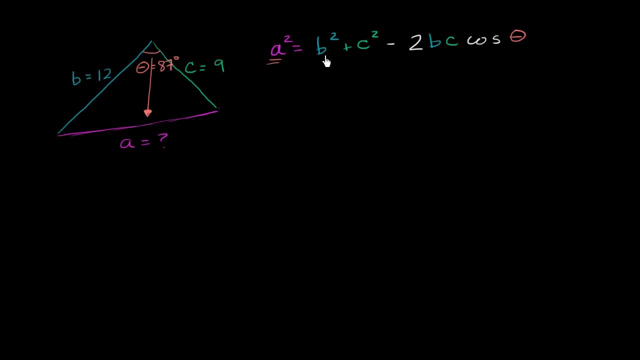 that we are going to solve for. So now let's solve for a, because we know what b, c and theta actually are. So a squared is going to be equal to b squared, So it's going to be equal to 144 plus c squared. 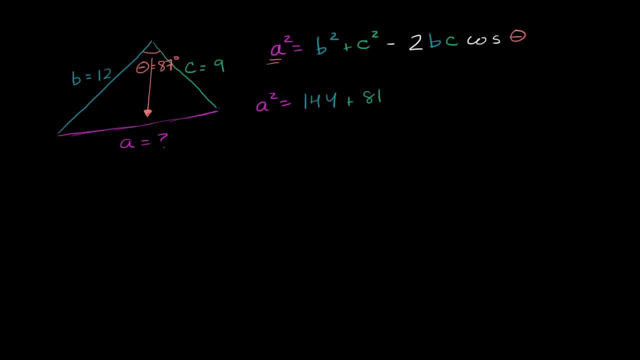 which is 81.. So plus 81, minus 2 times b times c, So that's minus 2.. I'll just write it out: Minus 2 times 12 times 9 times the cosine of 87 degrees, And this is going to be equal to: let's see, this is 225. 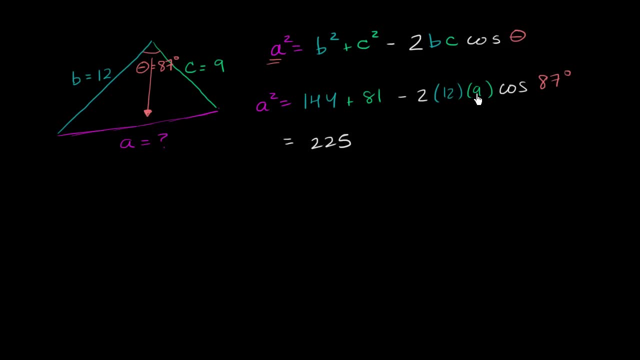 225 minus, let's see, 12 times 9 is 108.. 108 times 2 is 216 minus 216 times the cosine of 87 degrees. Now let's get our calculator out in order to approximate this, And remember this is a squared. 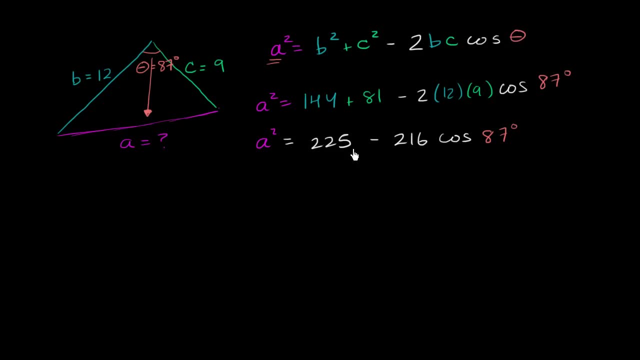 Actually, before I get my calculator out, let's just solve for a. So a is just going to be the square root of this, So a is going to be equal to the square root of all of this business, which I can just copy and paste. 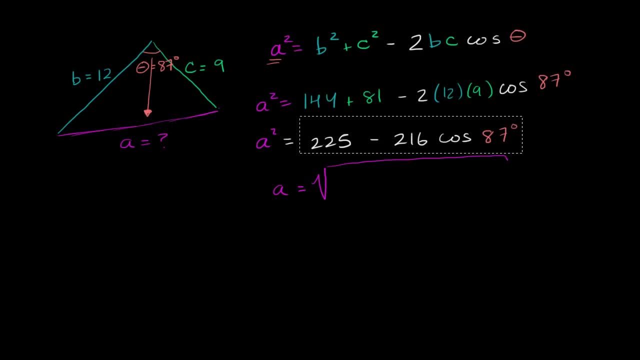 It's going to be equal to the square root of that. So let me copy and paste it. So a is going to be equal to the square root of that which we can now use the calculator to figure out. So let me increase this radical a little bit. 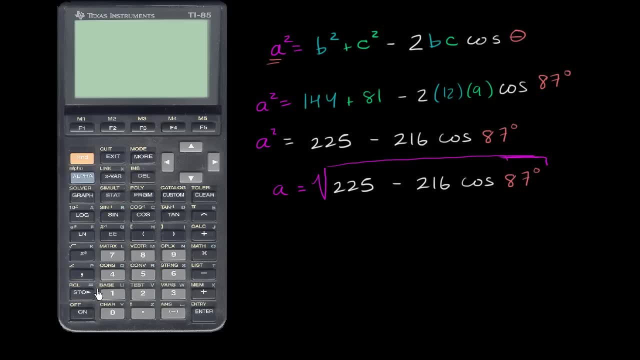 so that we make sure we're taking the square root of this whole thing. So let me get my calculator out. So I want to find the square root of 220.. Actually, before I do that, let me just make sure I'm in degree mode.